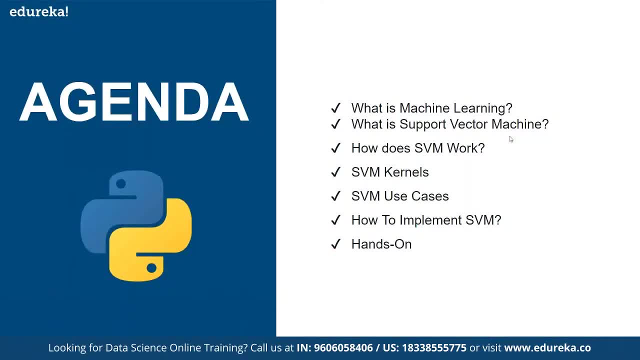 a great history which I'll share with you guys. Let's actually go into the agenda for the day. So before going into support vector machine, we'll do a brief introduction about what machine learning is, If there are some of you out there who are interested in machine. 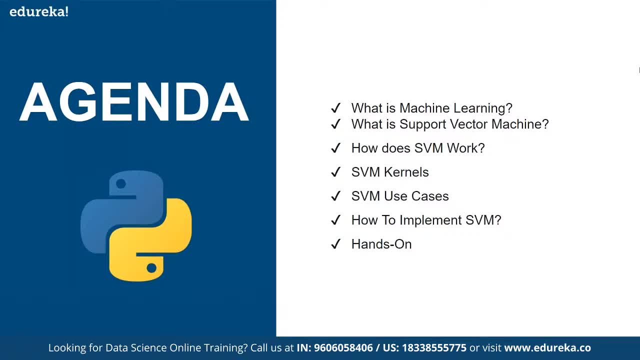 learning but don't know exactly what it is here. the buzzword everywhere that machine learning and deep learning and artificial intelligence, because in the next 10 years it will be something that will become very mandatory for everyone to learn, So it's better. 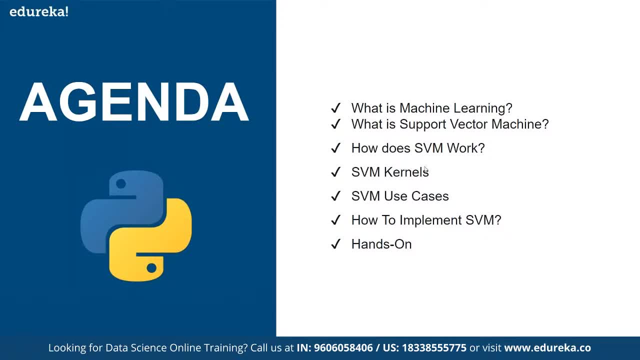 to get a headstart. Then we'll talk about support vector machines. Then we'll talk about how SVM works and what SVM kernels are, The different use cases that support vector machines have used, and we'll try to show you an implementation of SVM, If the time time permits. that's usually because SVM is. 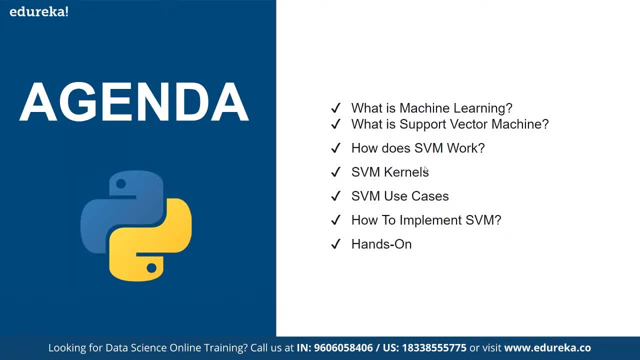 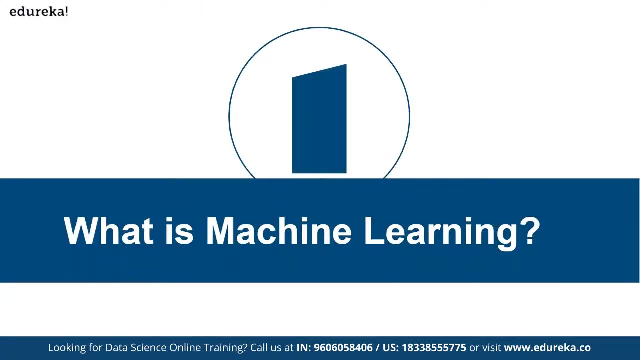 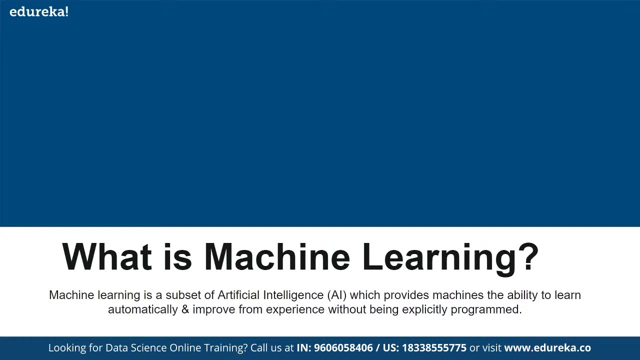 a longer topic. We might not find time, but I'll try my best to squeeze in some time for the implementation. Okay, So moving on first. uh, let us look at what machine learning is. So machine learning is a subset of artificial intelligence which provides machines the 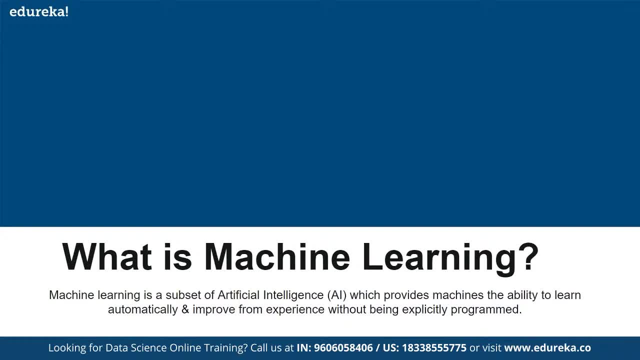 ability to learn automatically And improve from experience without being explicitly programmed, So you can think of it like the computer. to be like an infant. right, An infant has to be taught some things, So all the things that are taught to the infant is not based on knowledge. Some of the things 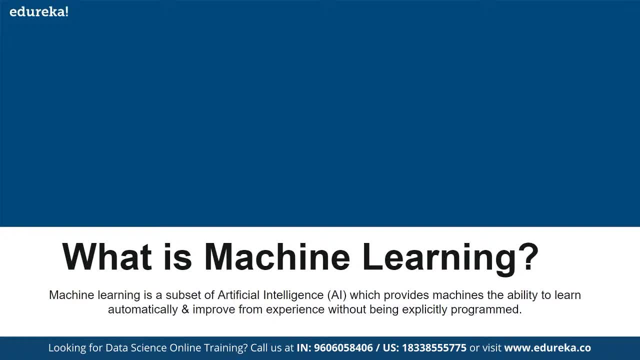 the infant will learn by itself. So when a child sees a fire it's gets attracted to the fire and the child touches the fire and understands that it will burn. So that is called learning. When I learn from some experience, from the data, similarly for a computer, suppose I'm. 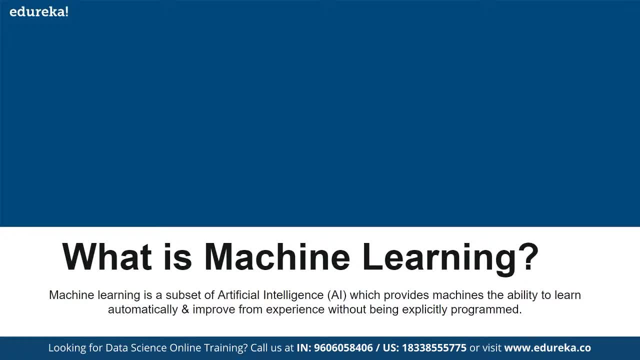 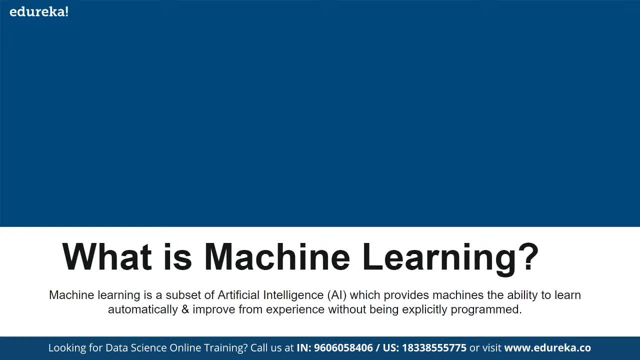 of the user. Based on that, we have given the computer that, based on some sort of financial data, uh, a decision has to be taken whether to give the person to go on or not. Okay, So that is what the computer will be seeing. 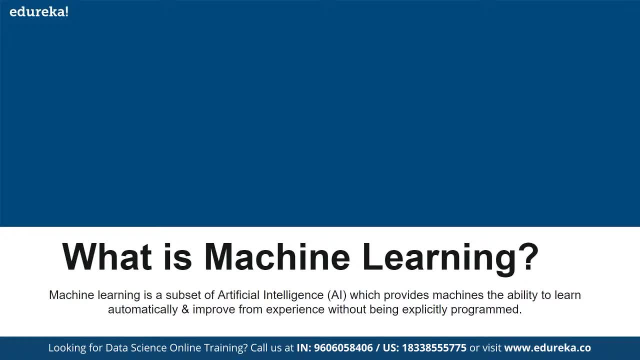 Said: okay, if the credit score is good, then typically we loan is approved. So that is what these machine learning algorithms learn. So we give them, these algorithms, some features to learn. So in order to make some prediction, by building a model- That is what it is called, So what a model basically is. 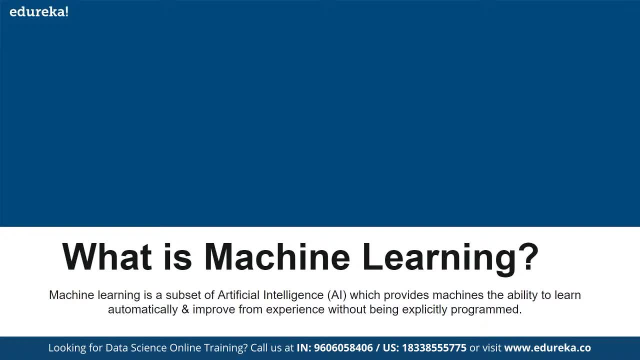 that based on the algorithm that I'm using. So machine learning has so many algorithms that are out there, And what we are trying to basically do is using these algorithms. we are teaching the computer set. Okay, So I have to decide whether to give a person. 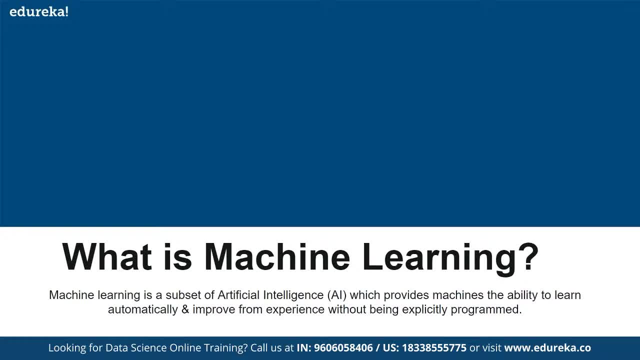 a loan or not. So how do I decide that, based on certain features- financial features of a person, The credit score may be, or past history, What sort of amount does the person have typically in his bank account? How much the person's salary is? So, so many things? 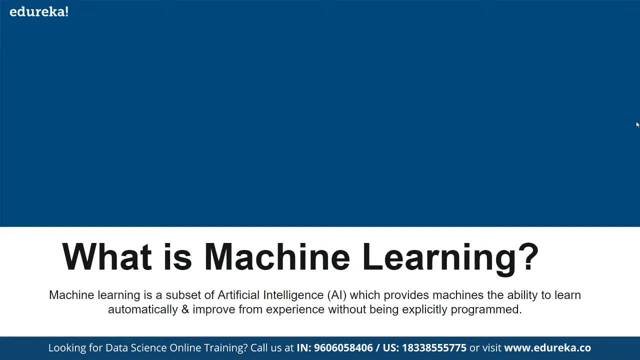 are there? So many things are thought of while deciding on something Right, And based on that, the computer will decide what to do. So it is building a model And there are so many algorithms to do it. svm is one of them. there are so many algorithms out there like decision trees, and then we have 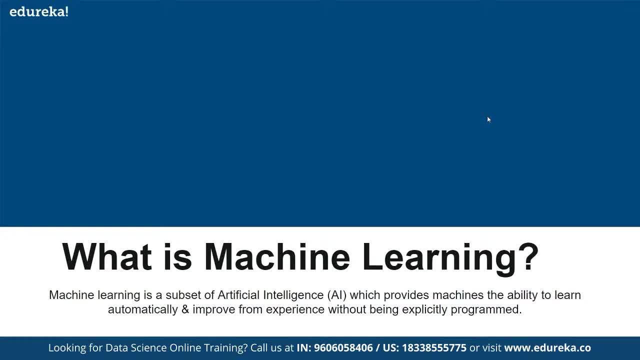 nine base learners, we have gradient boosting algorithms, we have random forest. so many algorithms are out there. svm is one of them and it is one of the best algorithms in machine learning. it came out late also, and we'll talk about the history of svm in some time and we'll understand. 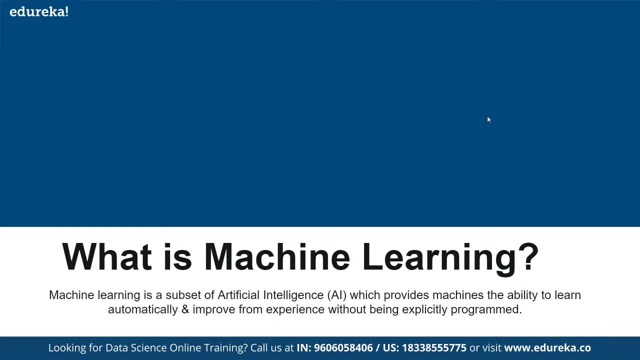 why it became very popular in the 90s, especially so this is in a. just what machine learning is teaching a computer, based on some already existing data, to take a decision. so if i give you another example, if i'm trying to predict the weather for in the next seven days, right, so what i'll do is 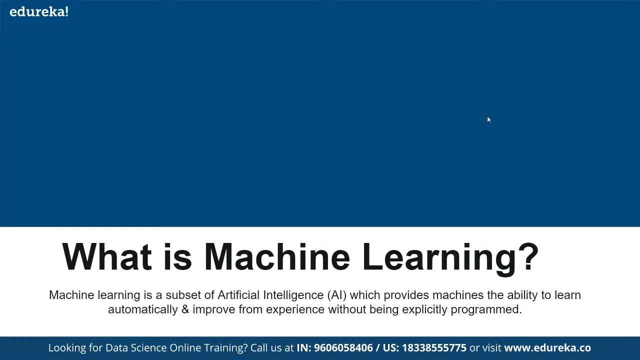 i'll see the weather for the last, say, 10 days. i'll see the weather on those particular days for the last 10 years maybe, and based on all this, i'll teach the computer to me. this is from how the machine learns in 2 Globes. so when you're teaching computer, 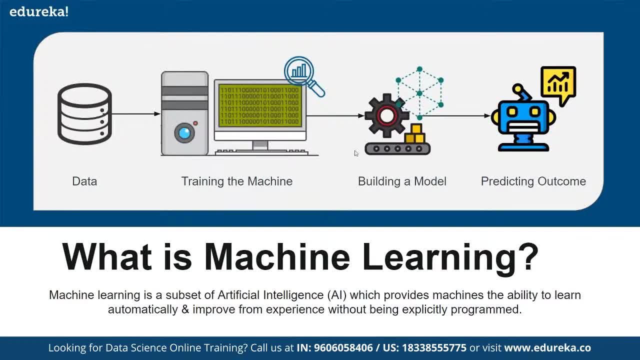 learning the computer and setting it up is the same, but now the computer can take a decision right. so this is what machine learning is. so what we essentially do is we have a data set, for example the lone data or the weather data. we are now training the machine, or teaching the. 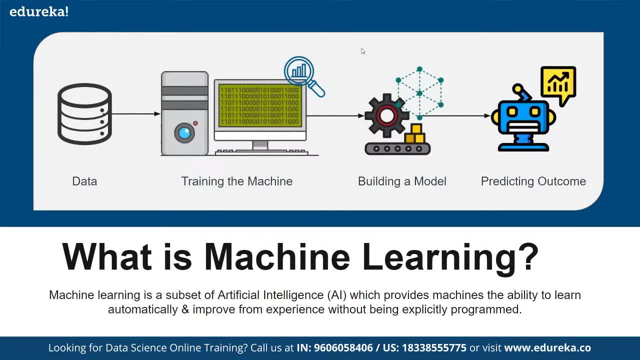 machine based on that data. if you have this type of data, then you should say: the weather will be cloudy, or maybe the person should. a new computer can program all that data into a learning input, the form in which, whatever the system learns, it stores it in a model. but i'll tell you, it stores. 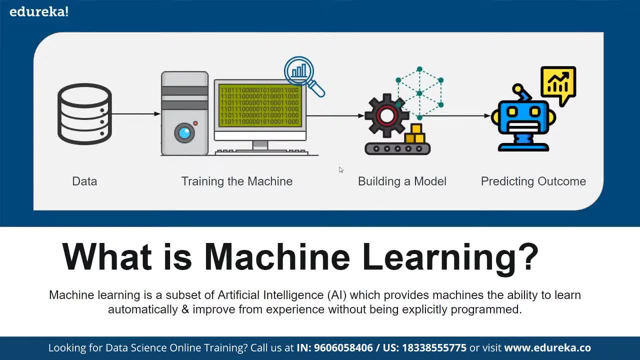 something called weights. so those are the things that are learned as part of this and then, based on that model, we predict the outcome. so this is how machine learning algorithm works. first i have data. based on the data, i do a learning. so suppose, as i took the example of an infant right, 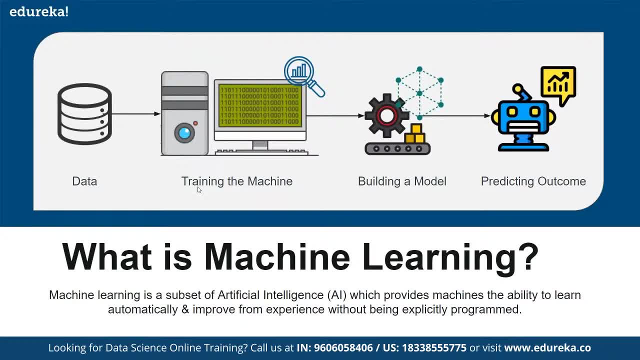 so the infant? there is fire, right. the infant touches the fire and understands that fire will cause a burning sensation that is stored in the model and then, whenever the infant sees the fire, the infant will know that if i touch it it will burn. so that is the predicting outcome. 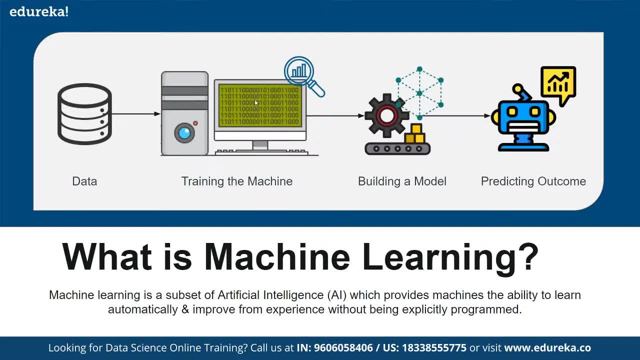 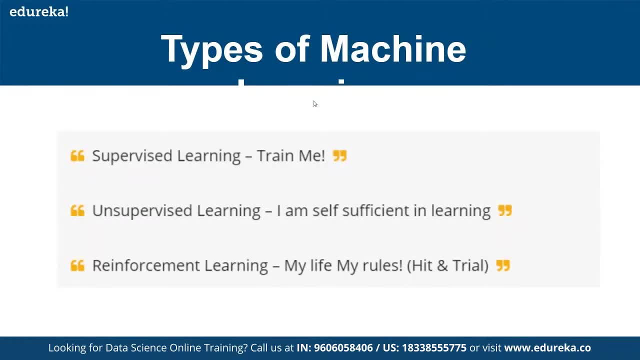 in the future, whenever the infant will see. okay, so that is how machine learning works. okay, so what are the different types of machine learning paradigms which are out there? first is called supervised learn, so whatever example i was giving you is supervised learn, so based on some data, and it needs to be annotated. or i should put in a way like: whatever the algorithm. 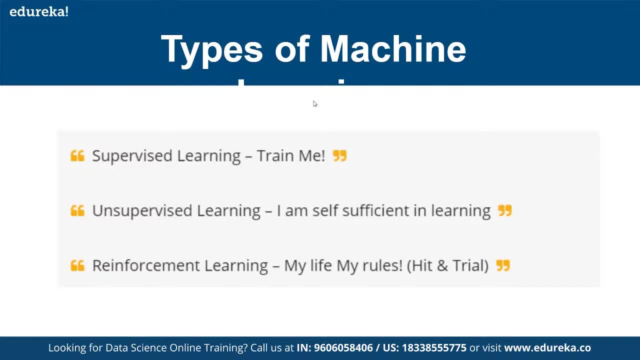 is trying to predict. the same sort of predictions are available as ground truth labels. initially, for example, when i'm learning to drive a car. right, so i'll learn that whenever i see a person or some to stop the car. okay, so that is what is being taught to me by my instructor. okay, when i'm 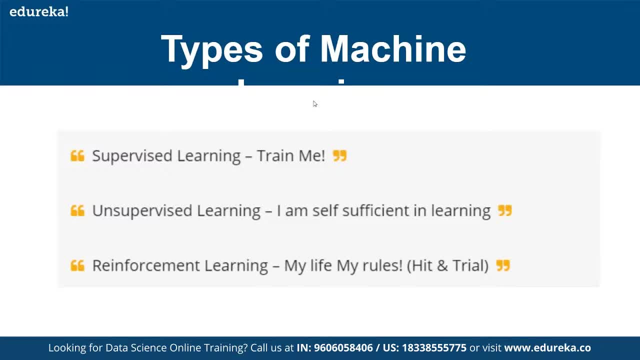 learning from an instructor. so let us take the example of driving and try to understand all these paradigms right. so when i'm learning from an instructor, when i'm learning from a teacher, the teacher will tell me: okay, there is an obstacle in front, so stop the car. so that is an annotation. 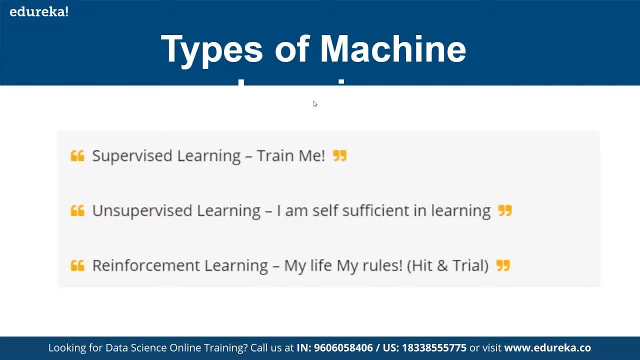 a label that is being given to me when to move and when to stop right. so i move. when there is no obstacle in front, i keep moving. when i see, say, a red light, when i see an obstacle in front, i see the person in front, i'll stop the car. that is what my instructor is teaching. so when i have 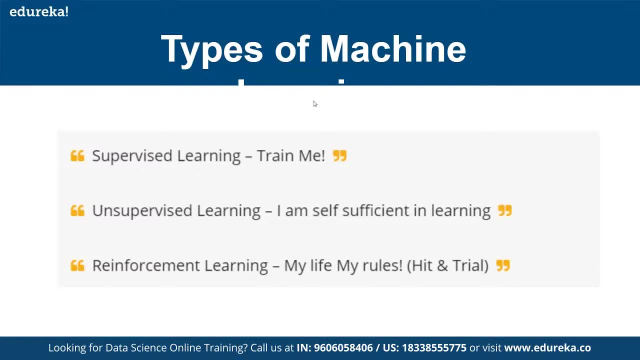 learned how to drive. i will know, based on what the instructor has told me, that whenever i see an obstacle or a red light, i have to stop, and whenever nothing of that sort is there, i'll start moving. okay, this is called supervised learning, because it is being supervised by a trainer signal or a teacher signal. okay, what is unsupervised learning? 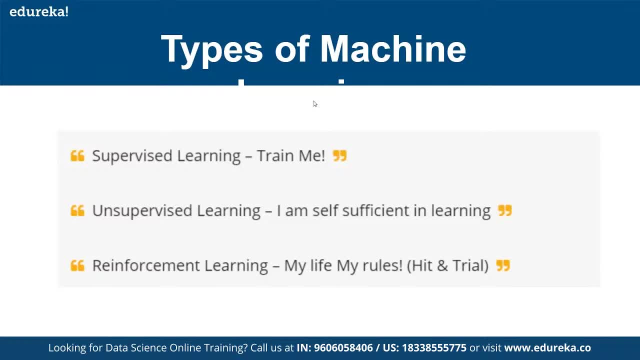 unsupervised is something where i don't have a teacher who is teaching me okay. so in unsupervised learning i am sort of based on whatever intrinsic values of data sets that are available out there. i am making a decision, okay, and say some sort of common sense is coming in. so as a human being, i have learned a lot of. 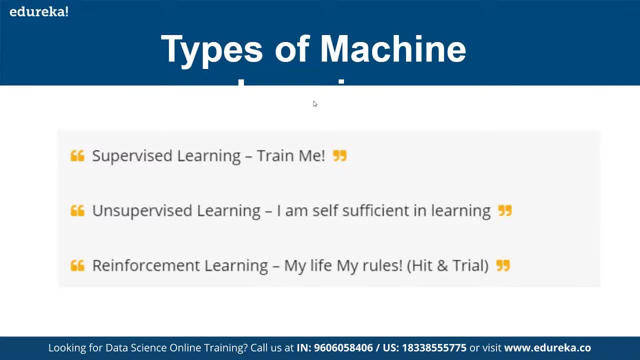 stuff before. so my knowledge, world knowledge, will come in. so when i'm so, i don't have a teacher. i started driving the car. okay, i know that there are things like the accelerator, the brake, the clutch and all these things are the steering is there, okay? so i've started moving the car and then i 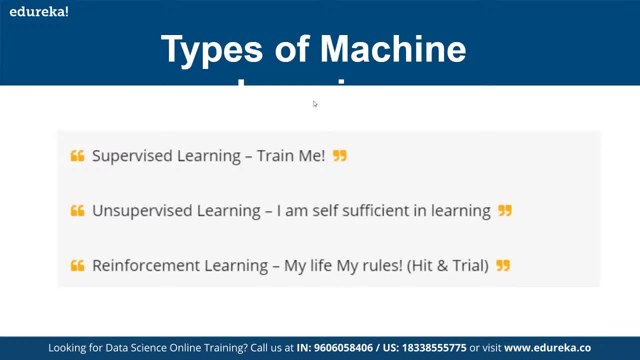 know that when an obstacle comes in front of me, i should ideally stop. i know if i don't stop what the outcome will be: my car will get hit. if there is a person, the person will get injured. right, this is based on some sort of world knowledge, so no one is teaching me based 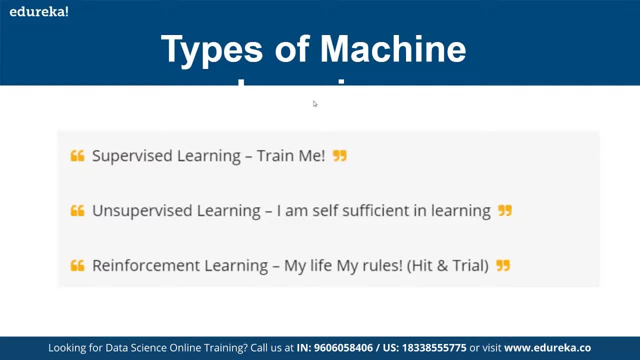 on intrinsic properties of the world that i already know. i am making a decision, so i am self-sufficient in learning that way. okay, what is reinforcement learning? reinforcement learning is: i have no world knowledge, i have nothing. okay, i just pick up a car and i do hit and drive. i. 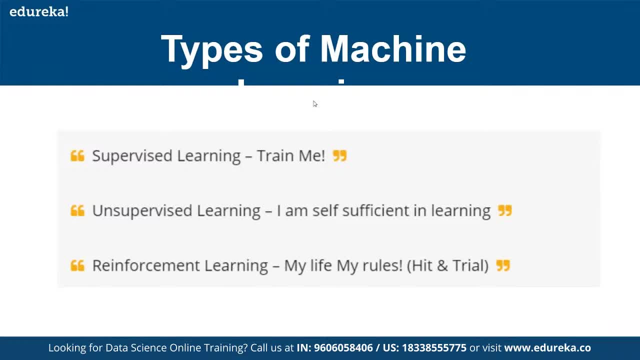 first accelerate and i hit it. hit an object, okay, hit a pole. so i understand now that if i hit a pole, if i see a pole in front of me, if i see an object in front of me and i press the accelerator, it will go and hit the pool right. so that is what i've learned from it. so it's hit and dry. so based 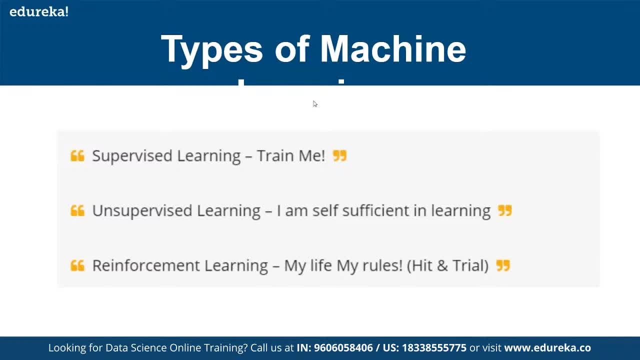 on experiences. there is either a reward or a punishment, right? so if there is nothing in front, i keep moving. i learn that. okay, so there is no obstacle in front, there is no person in front, there is no right in front, i keep moving. okay, i can keep moving. so that is my reward. what is my punishment? 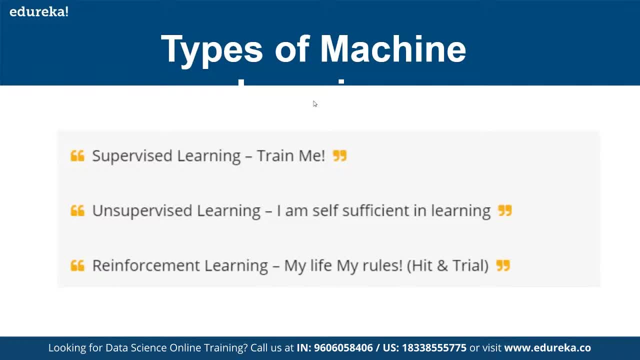 when i hit something, so that is how i learn. so reinforcement learning is very visible when you are training a puppy, for example. right, so when a puppy does the right thing, you give the puppy a reward. okay, so that is what the reinforcement learning means. these are the three major. 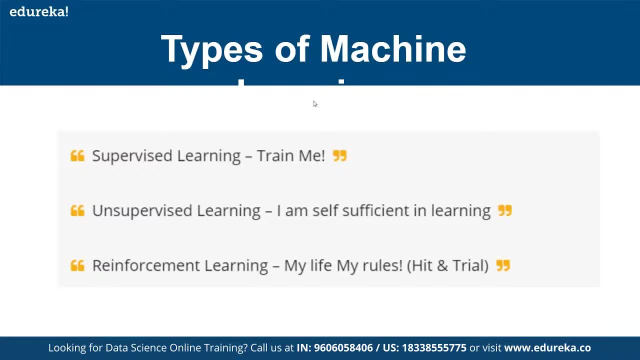 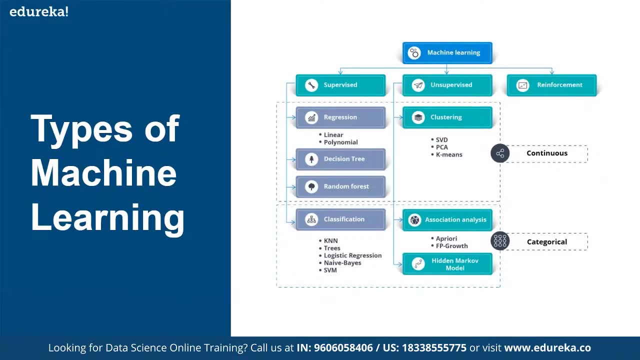 paradigms of machine learning. obviously they have sub parts. so, uh, to give you a broader view of what all of these mean. so supervised, if you go for the supervised part where a teacher signal or a trainer signal is involved there, right, so what we do is, uh, there are different types of problems. 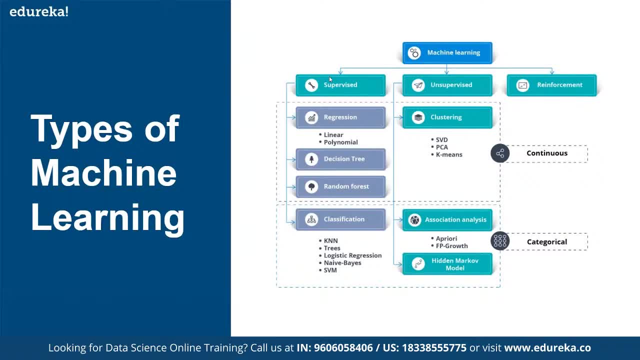 that can be solved using uh supervised algorithms. so couple of them are mentioned here. one is called regression and the other is called classification. so we have divided all of this into two categories: one is for continuous data and one for categorical data. so first you need to know what continuous data means. continuous means continuous values when. 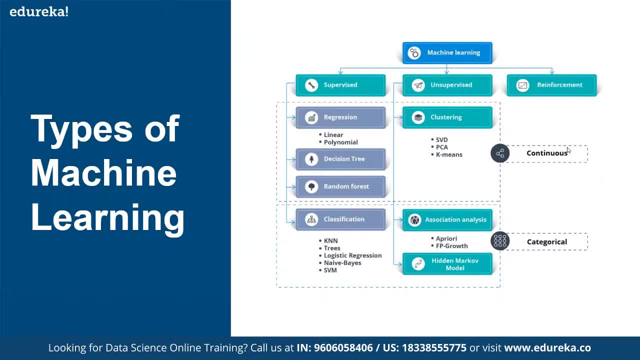 you are trying to predict a particular value, for example, we are predicting stock prices, right? so that is a regression problem it it does not have a category in which we have to put. so if there is a category in which we have to put it, it's called a categorical data. okay, for example, as i said, should 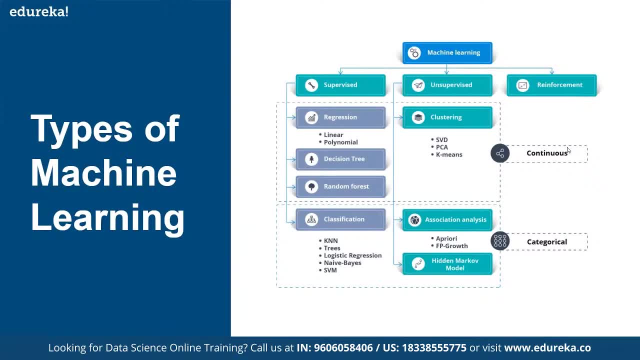 i approve the loan or not. should the loan be approved or not approved? yet there are two clear. so when i am making a decision based on some data that has been given to me, using a, the using a teacher, which is a supervised format of machine learning, it's called classification. 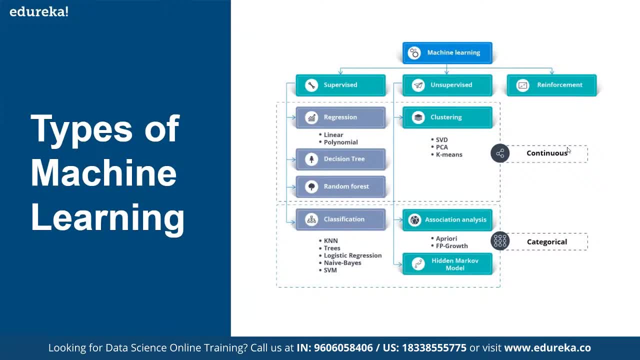 you are trying to identify the class in which the data should go: whether the person should get a loan or should not get a loan. these are the two classes. so, based on the data set available and the features available, i am taking a decision whether to give the first. 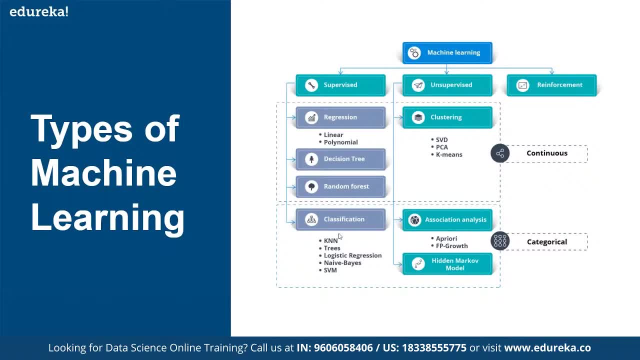 alone or not. these are the two classes. this is based on categorical data, okay, and continuous data means, as i said, when i'm trying to predict stock prices or, say, prices of houses in the neighborhood, okay, so that is called regression. we are trying to predict a value, not a class, not a. 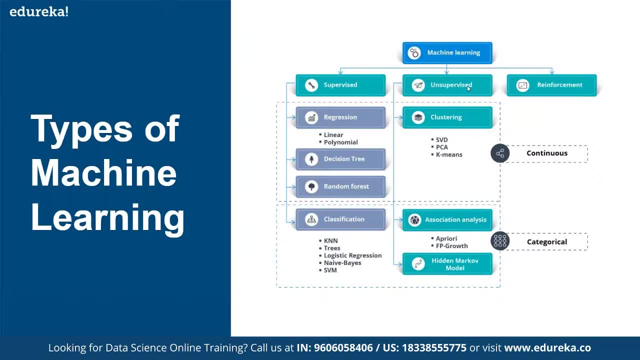 category, the same thing. uh, when i go into unsupervised, when i'm trying to put a data in a particular class without plan knowledge, using intrinsic values, what we are trying to do is we are clustering. so, in case of clustering, what is a very good example that we can take? so if we try to 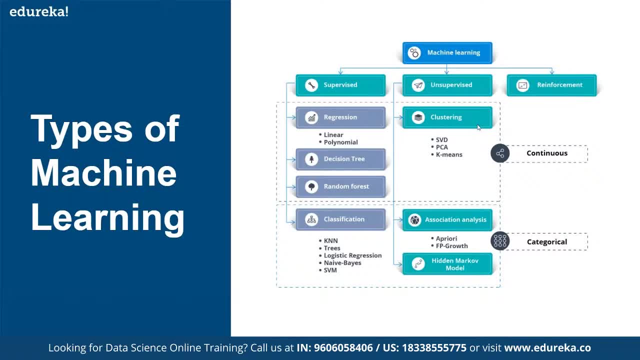 identify what seasons a day in the year will occur, right. so typically there are four seasons in a year, right, and we follow calendar for that. but if you use machine learning to identify which season a day of the year should go into right. so based on the weather in that particular day, we can call it. 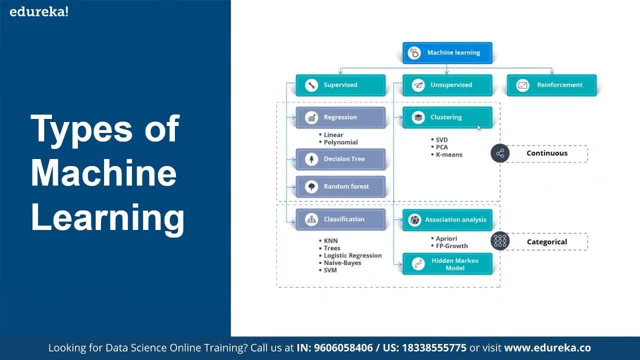 a day in winter or summer, spring or autumn, right. so that is clustering. so we don't need a teacher signal for telling us that, based on the features and the intrinsic properties of the weather of that day, we can classify, we can put that into a particular cluster or, in this case, we can put 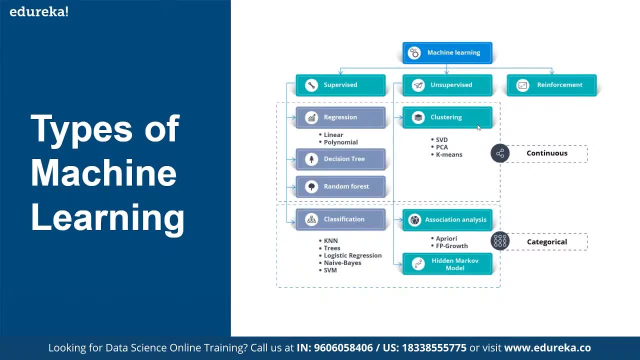 it into a bucket for a season, right? so, say, i want to find out the season for, say, fifth of july, okay, and uh, i have the data that it rains a lot. it's very hot in some parts, right, i'm talking about certain parts, uh, and and then what i can understand that it's. it should ideally go into. 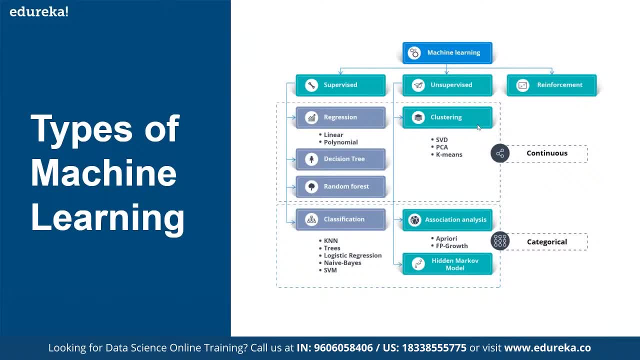 the summer bucket. okay, so that is how i'm clustering. no one has told me beforehand that. okay, so if this is the weather, it should ideally go into summer. no, this is just based on cluster. okay, based on what days are already there? so there are some. there will be some days in the summer. 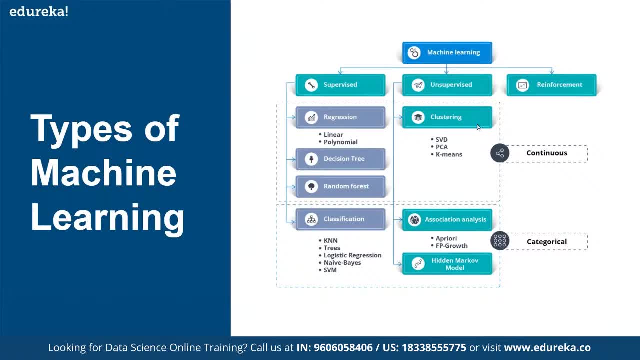 bucket already. so based on the intrinsic properties of the base, the weather, uh, the closeness to the other buckets, i'll decide where it should go. is that is called clustering for regression. there are different methods, like linear regression or say non-linear regression. polynomial is one of them. we use decision trees, random forest, even svms also is used for regression. 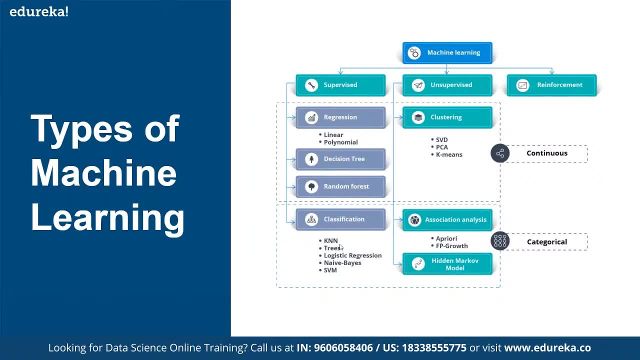 classification. there are so many algorithms. this bm is one of them. i've mentioned k, nearest neighbor, decision trees, logistic. so in this case logistic regression function is just used for doing the classification. it is more predominant in the regression part. then we have nine base, okay. so another part of unsupervised learning is called association. 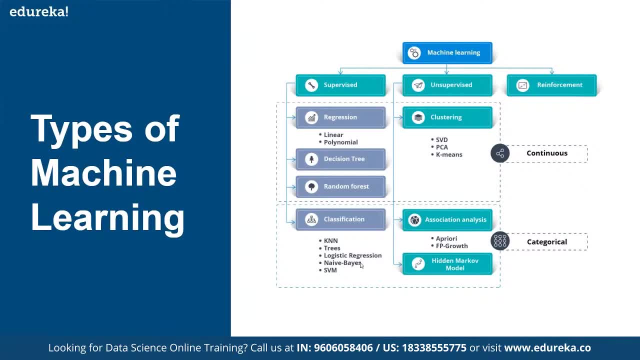 analysis algorithms like a priority or fp. so what is association analysis? suppose i have own a supermarket and i want to find, i want to place my items in such a way that it becomes easier for the people to access, thus increasing sales. okay, so putting bread close to butter, right, or say butter and jam close to bread- will automatically. 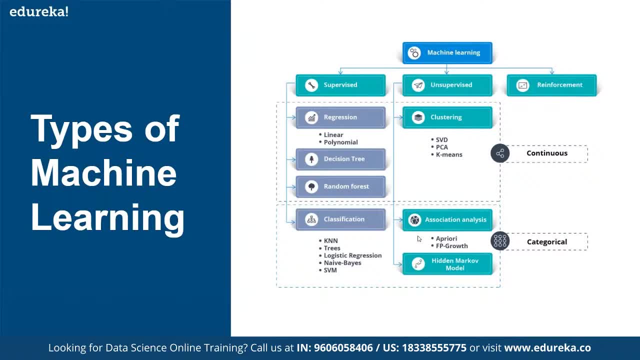 make it easier for people to buy that stuff, right? when a person buys a bread, the person will obviously think of buying butter or jam, right? so this comes from association analysis. what is the product associated with more? how is this found based on the buying pattern of users? what we are trying to do is we are trying to find out which products are. 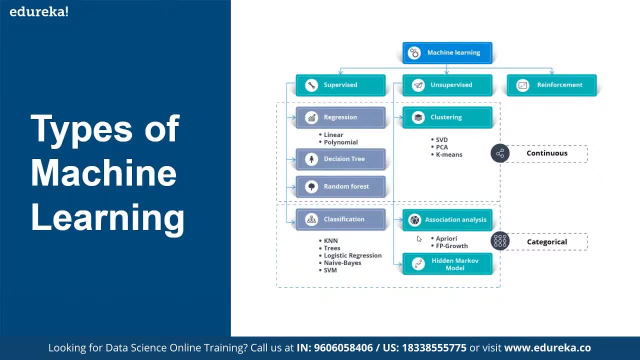 associated, associated more with each other. okay, bread, butter and jam are closely associated with each other. when i'm say, buying a washing powder or washing a detergent, right, so i'll be possibly buying a fabric softener along. so these are the thing that come through association analysis. okay. 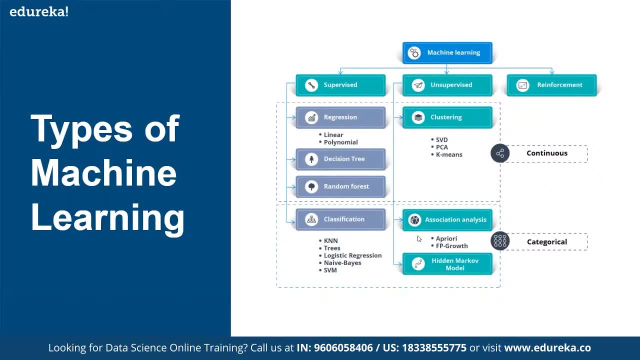 then we have something called hidden markov model. hidden markov models are part of a broader category of models called graphical models. so what these do is they sort of do some prediction on sequential data. okay, for example, i can say say, say for time series analysis, okay, like weather prediction over the. 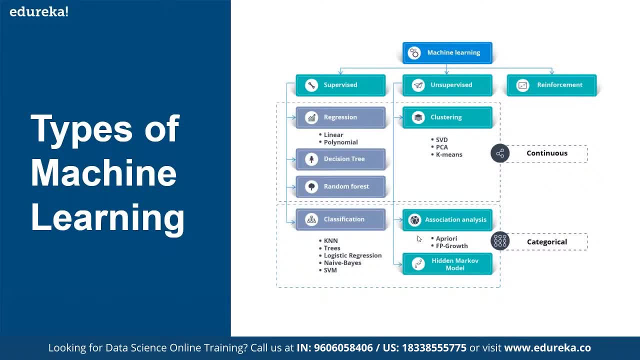 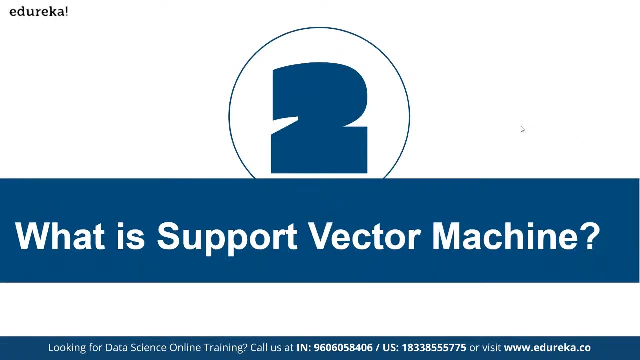 last 10 days i had some sort of weather. what should the next day of the weather, next day, what sort of weather should be? so these are called sequential data, and hidden markov models are used for predicting sequential. now let us talk about support vector machine. so this is: 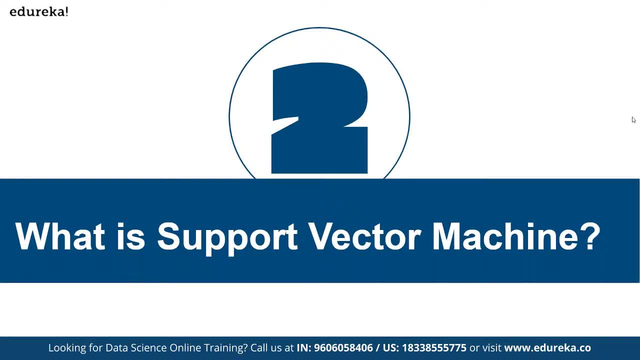 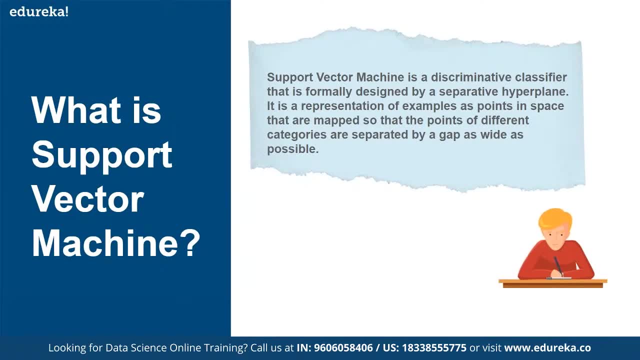 like i was talking about decision trees and k nearest neighbors and naive basal garden. so this is the formal definition of a support vector machine. it is a discriminative classifier that is formally designed by a separative hyperplane. it is the representation of examples as points in space that are mapped so that the points of different 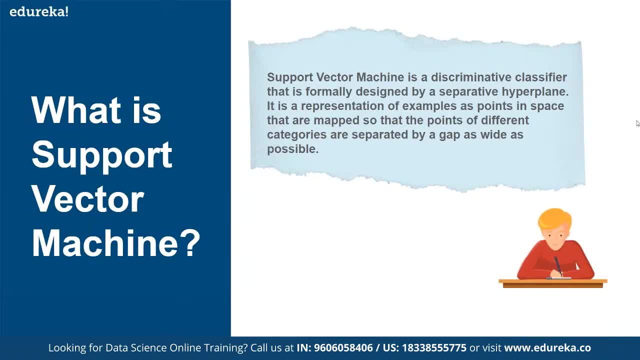 categories are separated by a gap as wide as possible. okay, so this is what is the formal definition of support vector machine. okay, so if you don't understand this, that is understandable. okay, so i'll sort of try to explain what this definition is. first of all, it's a classifier, okay. 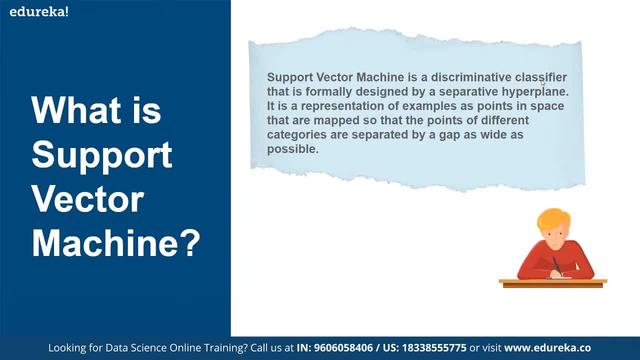 it's a classification algorithm, as we saw in the previous case. right, there is a part of supervised paradigm of machine learning called classification. so what we are trying to do is we are trying to do here is we are trying to identify a class. okay, what bucket should the data go into? whether the 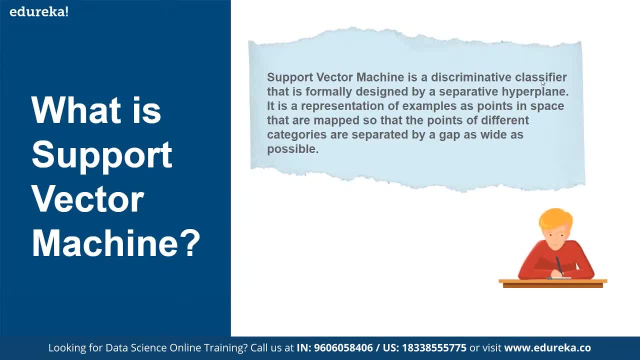 person. person should get a loan or should not get it. okay, so, uh, that is called a classifier and it's called a discriminative, because, based on the features, i'm trying to predict the class. there is another mode of machine learning algorithms, called generative, where, based on the class, i sort of predict the features. it's the other way around, okay. so. 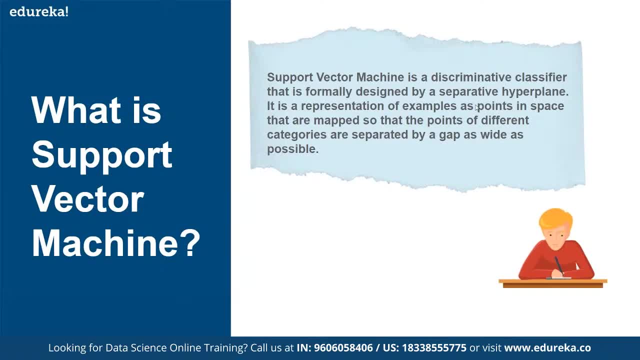 so it is. the difference that svm creates with other machine learning algorithms is that it creates a separative hyper plane. so in classification what we do is, if we have the data points projected into a particular space, in a particular, say, three dimensional space or two dimensional space, what classification algorithm tries to do is: 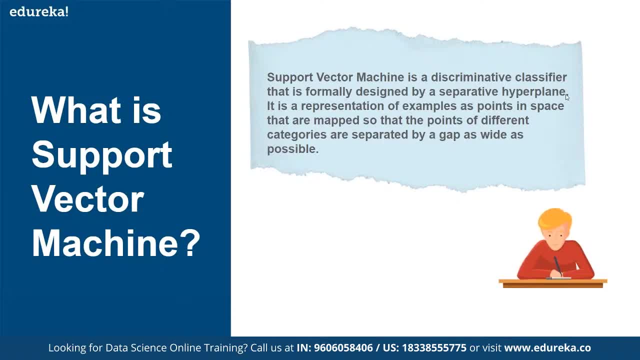 it tries to draw a boundary between the classification points. okay, we'll see in some time how that actually works. but, uh, what svm does is it will create a space. it will create a sort of- uh, separating space between the two classes. okay, so that is the distinguishing point of 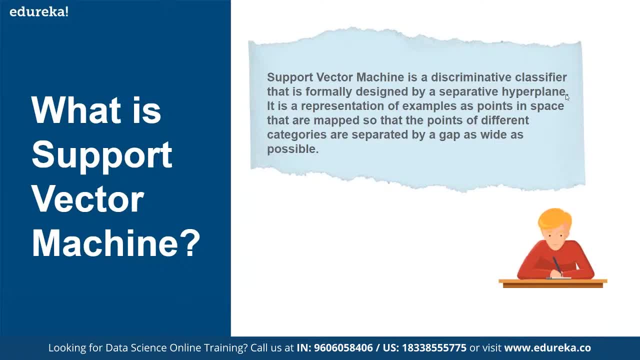 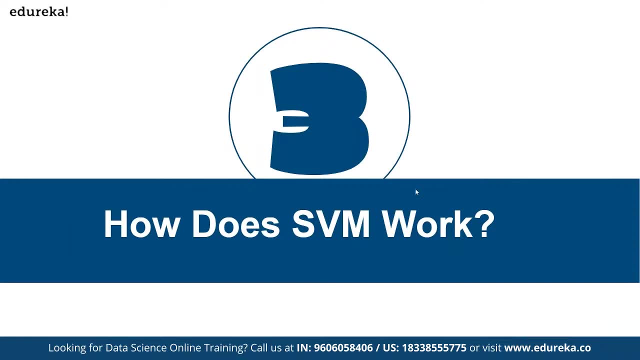 svm, and another distinguishing point of svm is called an svm kernels. that is what we will discuss. okay, so before going into how svm works, i'll quickly discuss in short how svm came into existence. so this russian computer scientist named vladimir vatnik, so in 1963 he published his 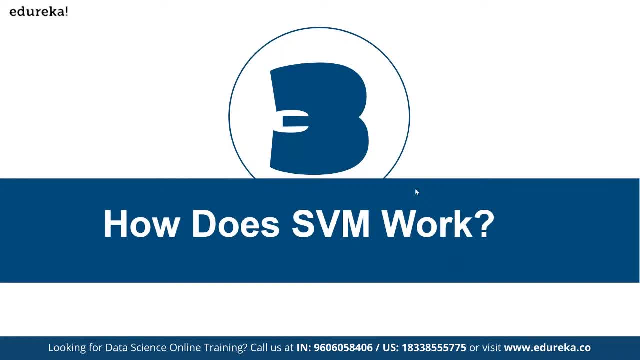 he submitted his phd thesis and he got it published in in russia. so in 1963 he had thought of svm. okay, he has not. he thought of a separating hyperplane between two classes for classification and golf. it was as early as 1963.. so post that, people thought of k-nier, sneakers and decision. 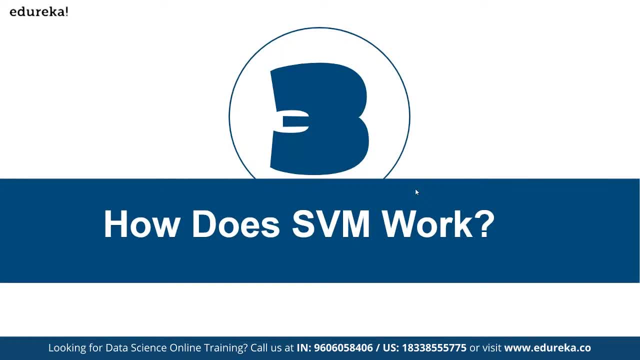 nine base algorithm based on Bayesian probability theorem. so he came to us in MIT in 1990s and the problem with establishing how powerful SVM was that he didn't have the tools to do that click. now we have a powerful machines to run algorithms right. so that is one of the reasons why deep 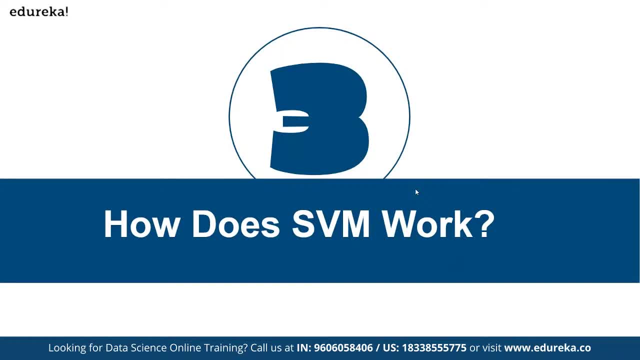 learning came into the forefront very late. now we have powerful GPUs to run complex algorithms over months in some cases, so that computational power, once it came, then deep learning, came into the forefront. at that time, just imagine there was nothing, that there was no computer, there was nothing. and in 90s again, the sort of data set that he had, the huge set of calculations that 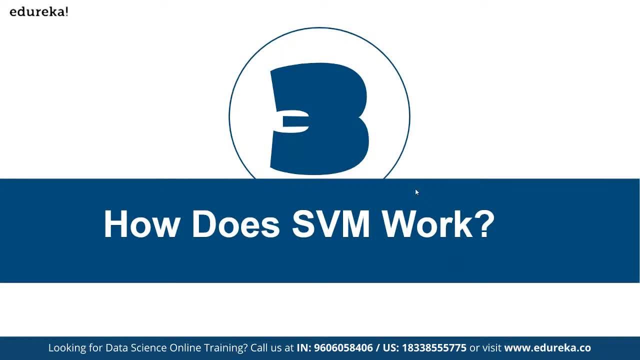 he had to do to establish how powerful SVM was was, again, not this. So what he did is he went to the numerical analysis people and asked them to do some sort of estimation based on how powerful it might be. So it included a lot of calculations and numerical analysis. people were actually department. 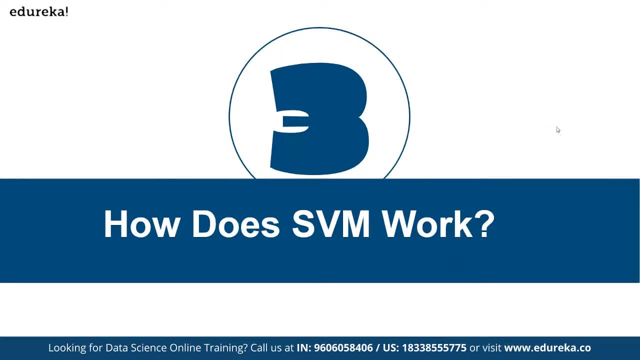 where people used to go for complex calculations and all. So this was in 1992.. And 1992 Vapnik could establish how powerful SVM was. So it's like 29 years after he had actually come up with the idea, people came to know how powerful SVM was. 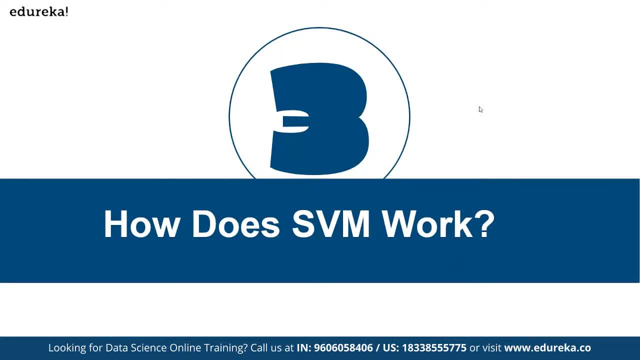 So SVM became very popular because of two main concepts. One is the base concept of SVM of creating a separating hyperplane, and the second concept is the kernel concept of SVM. So SVM is the kernel concept of SVM, So SVM is the kernel concept of SVM. 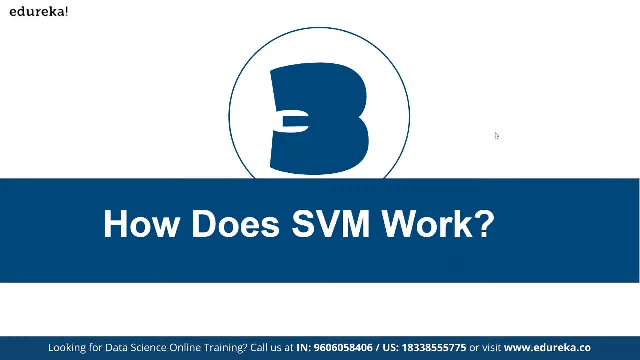 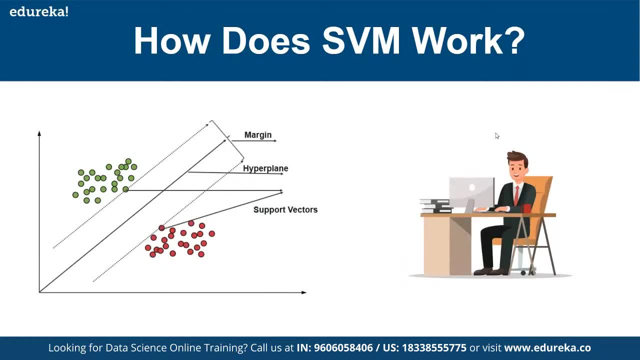 Which, and both of which we'll be discussing shortly. Okay, so how does SVM work? We have been talking about something called a hyperplane, Separating hyperplane, So first let us understand what classification is. So, say, I have a data set of people. 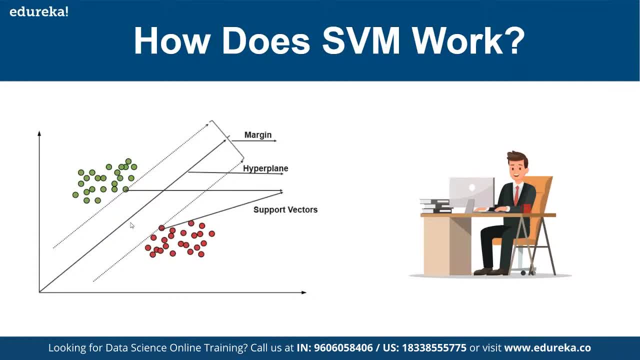 for whom loans have been given and some data set for people for whom the loans have been denied. So, whether to give a loan to a person or to deny the person a loan- See the green dots over here are for cases where the person has been approved the loan. 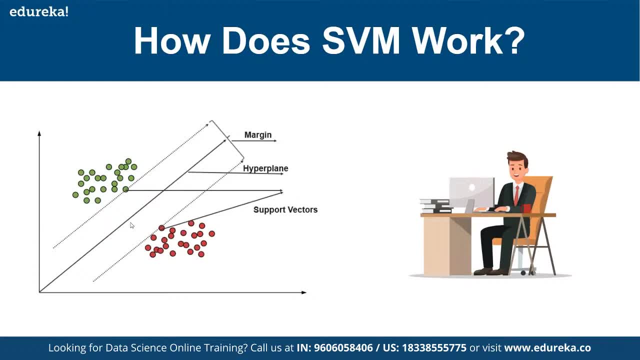 and the red points are cases where a person has been denied. Okay, so you can see, on a two-dimensional plane, on a two-dimensional projection, These points are clearly separated. Okay, this is an ideal situation, and what my classification algorithm is going to do is that it's going to be. 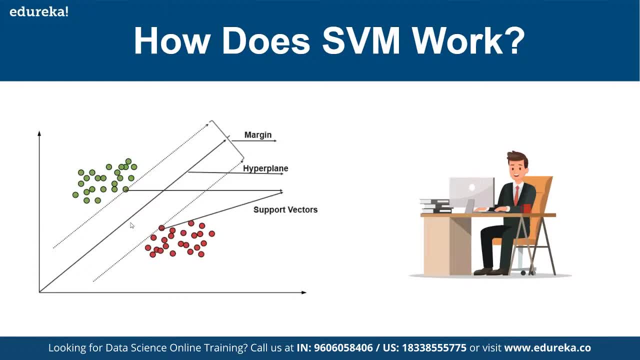 will do is it will create a separation line between both of them. So why do we need to do this? Why are we trying to do this? We are trying to do this for a prediction. Okay, as I said, so, this is the data set that has been given to us. 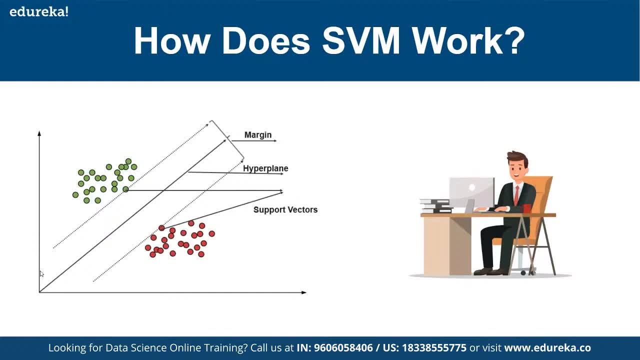 The algorithm has gone through some training and learned that, okay, these are the points which are for loan approval. These are for loan denial. Okay, and based on that, it is create a model. Is it has created a model? So what is the model? 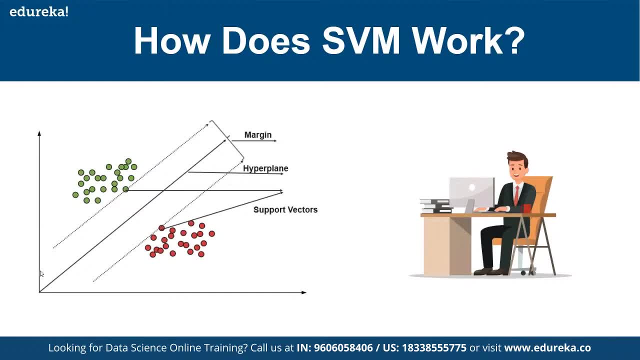 It has created a separating line between the two categories. So, be it decision tree, be it random forest, be it nine ways, be it neural networks, be it k nearest neighbors, all algorithms will try to create a boundary between the two data sets. 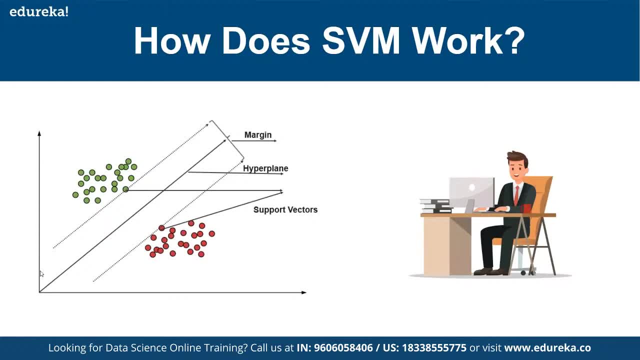 Okay, that is the aim of classification. So why do I need to do this? I need to do this because, for example, if I have Another point that comes here, okay, So I don't know what this point is. So this is a set of features that have been mapped here. 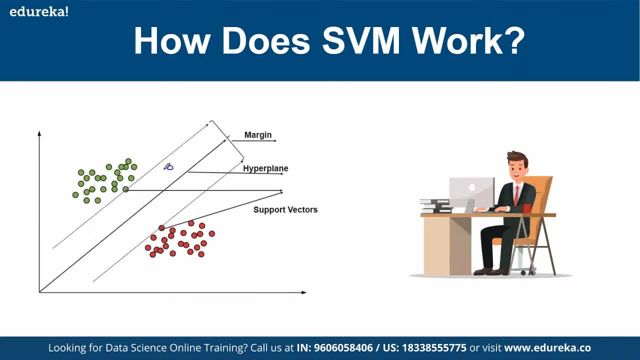 for a new user has come and I don't want the people at the bank to decide whether to give the person alone or not. I want to do this automatically using a machine learning learning. So there's a point over here. So how do I decide it? 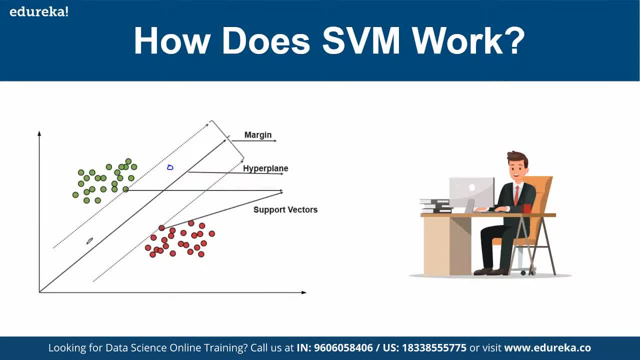 My separating hyper plane is my separating line, my classification line. The model that the algorithm has learned- machine learning algorithms has learned, based on the data set that has been provided- is this one. So it is on the upper side of this line, So this is closer to this. 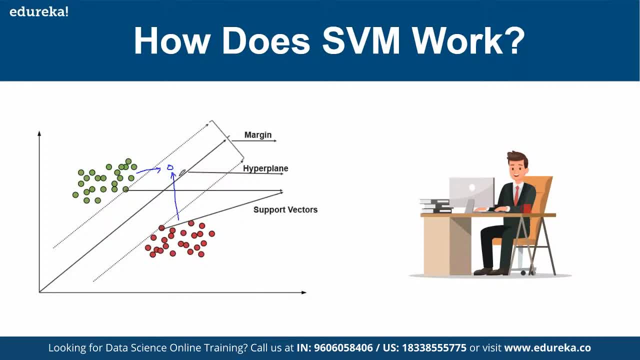 Rather than this right, ideally, and it is on the upper side of this line, Correct. So what I'll do is I'll tell to approve the loan because it is near to people who have been approved it And on the on the upper side of this classification boundary that I've created. 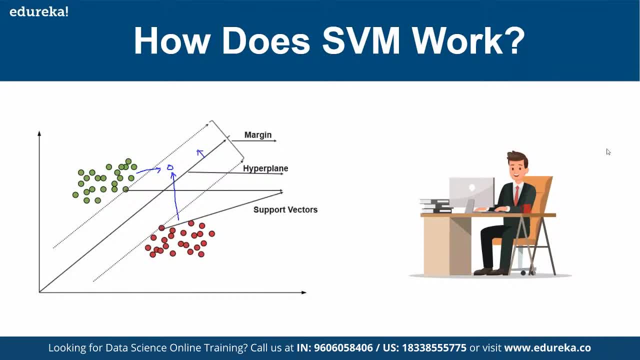 Okay, this is what typical classification algorithms do. Okay, So now, what does SVM do differently from these classification algorithms? SVM does not draw a boundary like this. What it does is in two-dimension. Let us think of it in two-dimension. 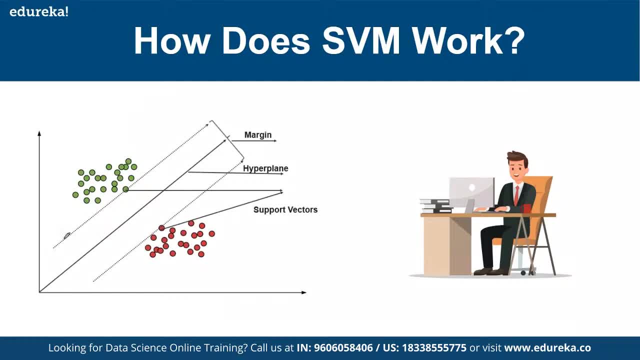 What SVM is trying to do here is it is trying to create a boundary between these two points. So I'll try to create the farthest boundary between these two points, So I'll see which is the nearest point to this boundary. This, it is this point and this point. right? 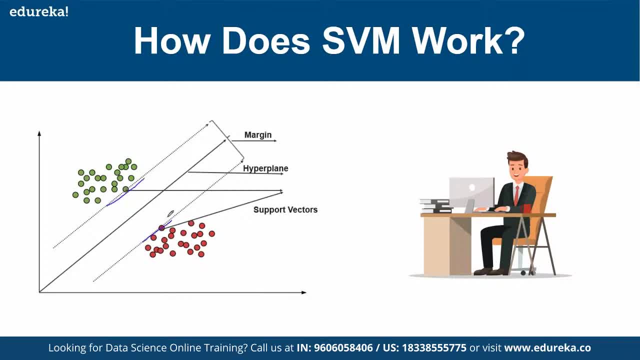 So I'm creating a boundary from here to here, both passing through these two points. So this is what is meant by a separating hyper plane. So hyper plane is in n dimensions in case of two-dimensional. in two-dimension, It will be separating lines in case of three-dimensional. case data set. 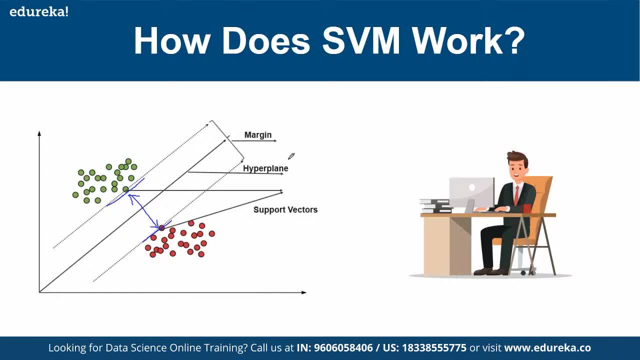 It will be a separating plane and in n-dimension It will be separating hyper plane. Okay, so a generalized version would be separating hyper plane. Okay, So this is the separating hyper plane that I'm drawing, and these two lines which have drawn are my support vectors. 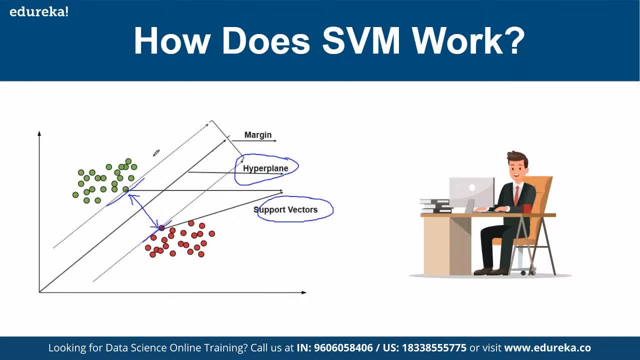 And my separating hyper plane is this one. So over here, The equation of this line would be plus one- Okay, this would be minus one And this would be zero. Okay, I'm trying to find a middle or a mean between these two lines. 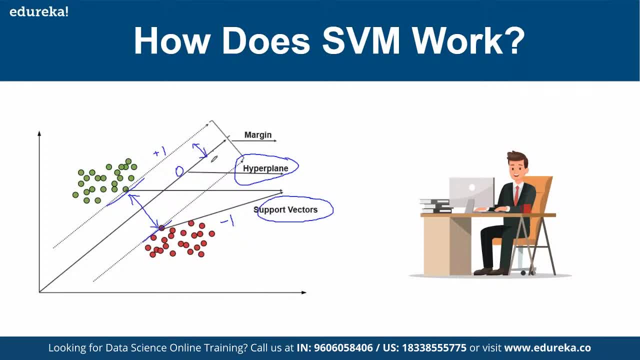 Okay, so this distance And this distance would be same. So, first, what I do is: First I try to create the separating lines. This is the step One that I'm trying to do. Okay, I create the support vectors first, then 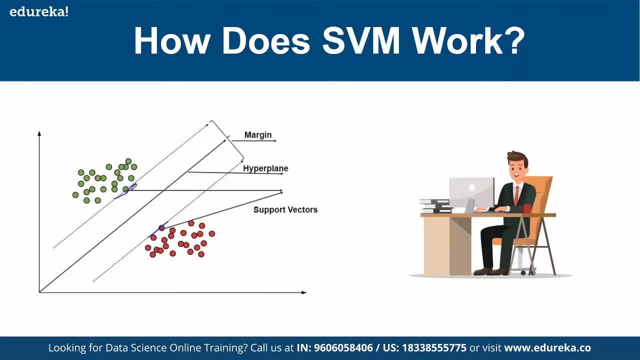 How do I create the support vectors based on the data set given? I'll find this farthest distance, Okay, between the two data sets. This is the aim of SV. It will try to find the farthest distance between the two data sets. 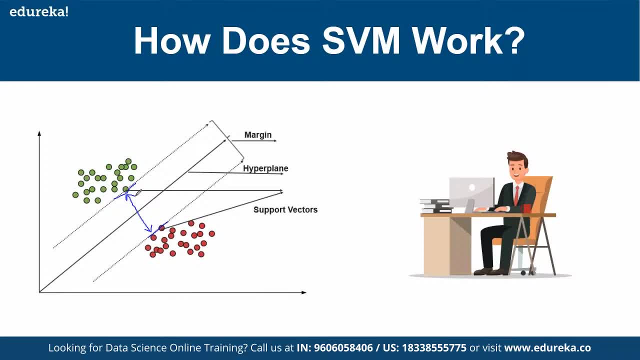 So it's creating, say suppose you go to a zoo around the Tigers Arena, There is a big moat right And the moat is made as big as possible So to separate the tiger from Tigers from the human. So what I'm trying to do is from this data, from the positive data set, 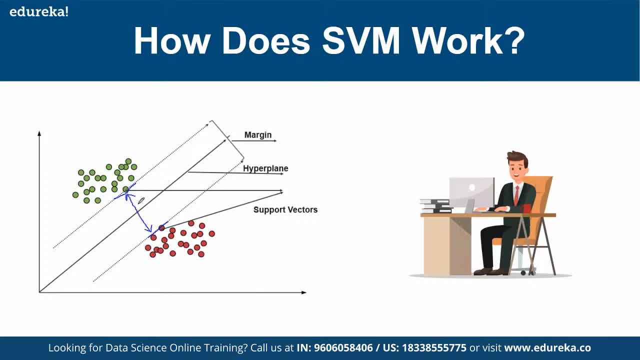 and the negative data set, I'm creating the farthest distance. Okay, so these two vectors which pass to the farthest point between the two data set. So farthest point means this is nearest to this one, This is nearest to this and this is nearest to this, but it is farthest from each. 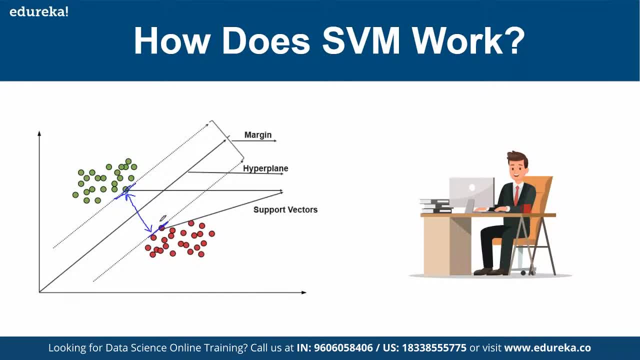 Okay, This is okay. I'm sorry, It's not far. This is the nearest point, the nearest data points to each other. That is where my support vectors would be created. This is step one. step one is creating the support vectors. Once these support vectors are created, 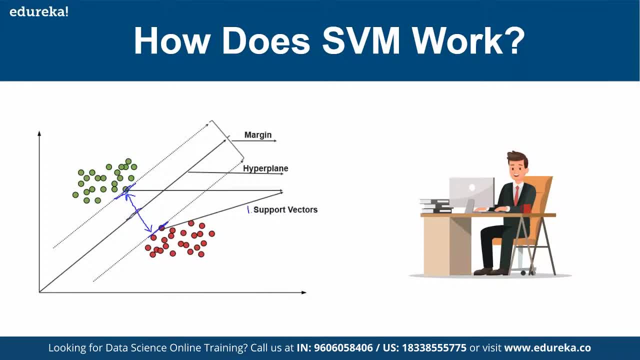 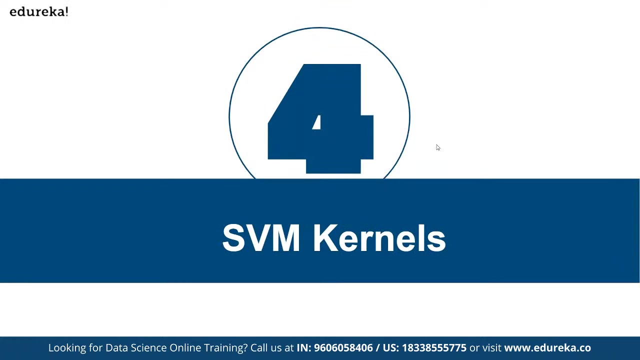 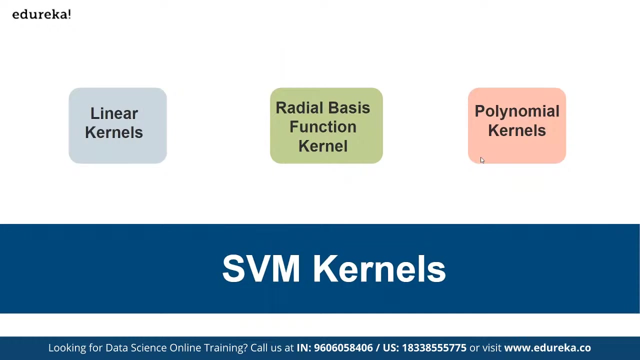 I take a perpendicular bisection of this and create this line which is called my hyperplane. and that is step two. Okay, Just to make sure we have the right. So if you look into the SVM library of SK, learn There are linear kernels. 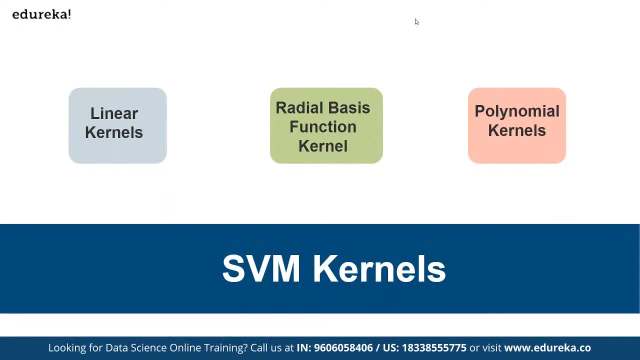 So these are just linear transformation of points into another space. linear transformation, radial basis function would take it into it by theta sort of transformation. polynomial kernels is using polynomials to transform the two-dimensional polynomial, three-dimensional polynomial. So these are just transformation function of points into another space where the separation 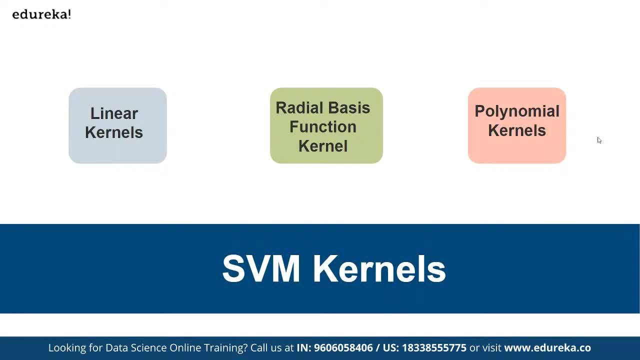 becomes easier. So the point is, the separation might not always be linear. We might not always be able to get a line to separate these points. Sometimes we need a nonlinear separation. So for that we need nonlinear kernels like radial basis function or polynomial kernels. 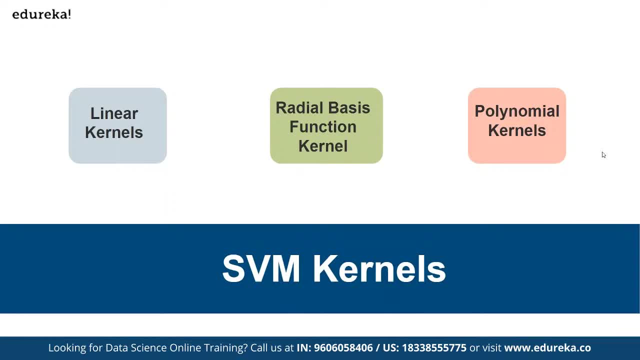 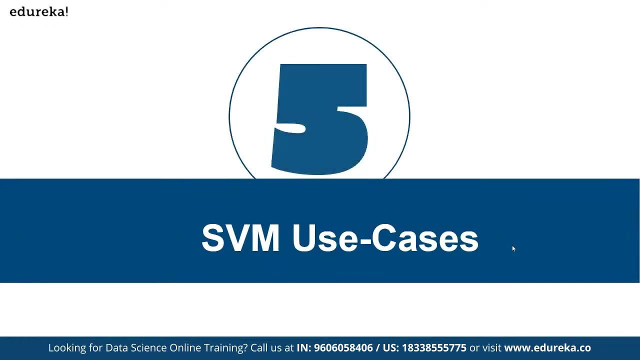 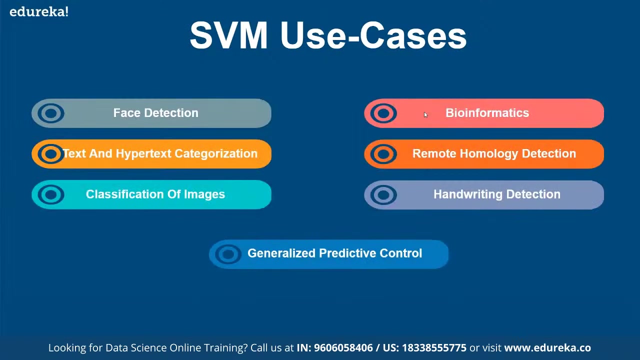 Okay, There are some other kernels, like a Fischer kernel, and say Gaussian kernel. Gaussian kernel is sort of a normal distribution curve, So do transform the functions using a normal distribution. Okay, what are the use cases in which we apply SVMs? So if you have seen these applications out there- face detection, text and hypertext categorization- 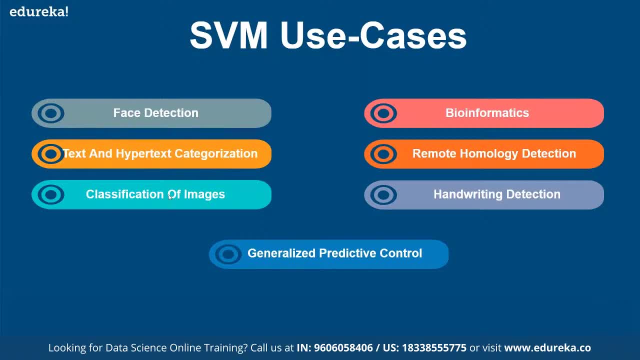 classification of images. so images image classification is like I want to identify an image contains a cat or a dog, So that sort of those. again It's classes, and I've given, I've been given, say, 10,000 images of cats and dogs to train. 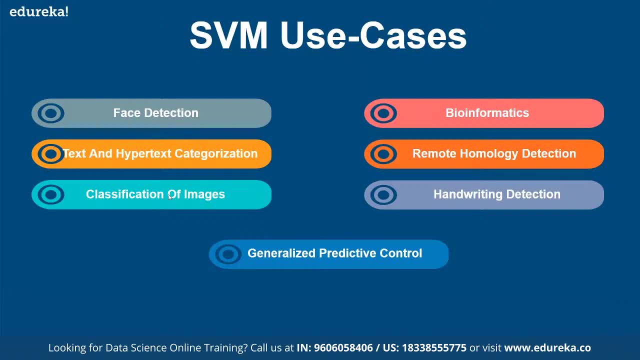 on and teach the system to draw the support vectors and then correspondingly the hyperplane. So in a new image comes, based on whatever I have learned, based on the hyperplane that I've drawn. I'll try to find out if it, on which side of the hyperplane, on which side of the decision. 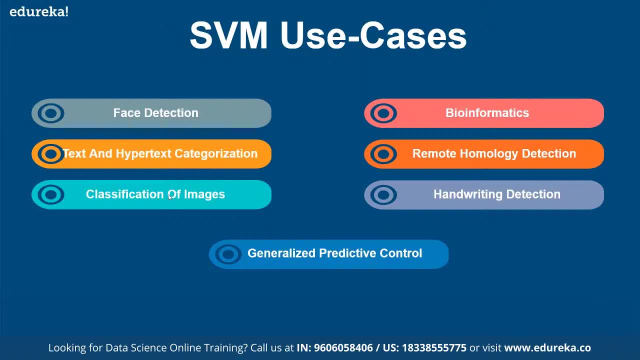 boundary. this new point occurs based on that and we making the classification. in bioinformatics It is used Remote homology detection, handwriting detection, So whether a particular handwritten character is an E or a B, so we'll have 26 classes in that case. 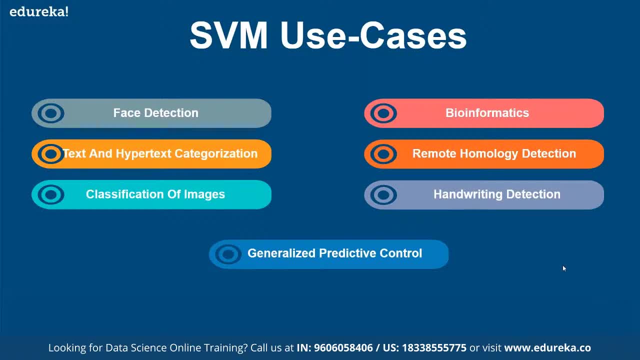 Okay, so this is a multi-class classification problem, So in fact any machine learning algorithm can be used here. but SVM is a really powerful case because of two factors: One is the separating boundary concept- Okay- and second is the, the kernel case, right there. 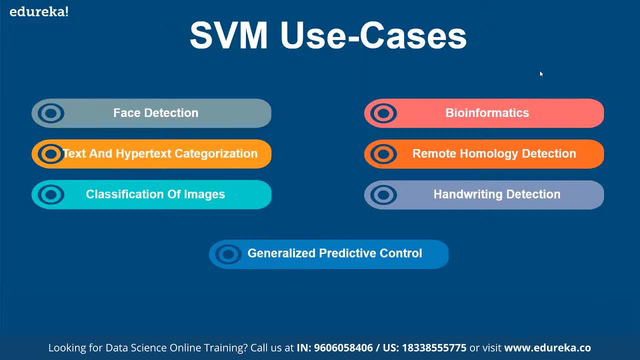 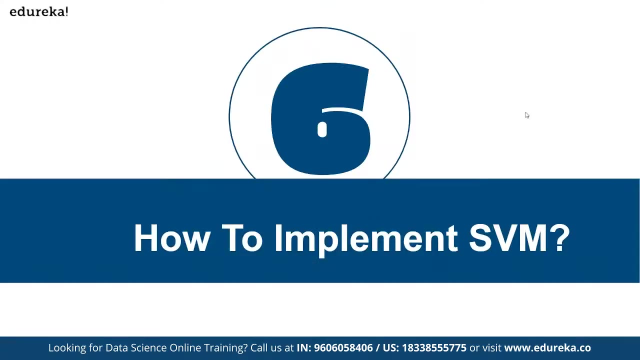 It can transform The entire data set into a different dimension and then the separation become between the two classes becomes easy, generalized predictive control. So these are the different domains in which SVM is used. Okay, how to implement SVM. So this is typically same for all machine learning algorithms. 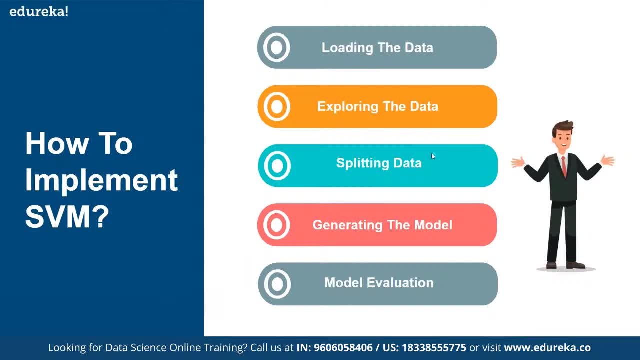 So we load the data first, explore the data, split the data into training and testing. So we use the training to acquire the knowledge and testing to test the knowledge that we have acquired. So, based on that, we keep tuning the data set, keeping the parameters, keep changing the kernels. 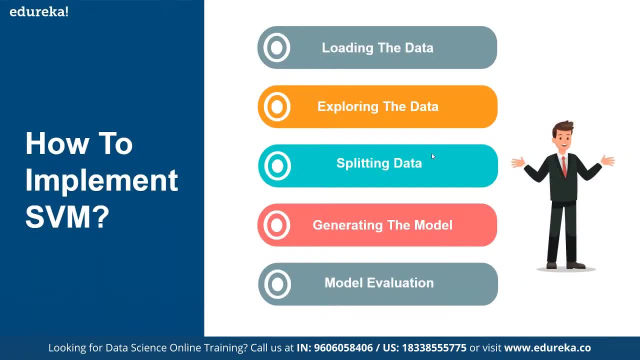 So, based on that, we can improve the accuracy of the system And then, finally, we generate the model and then evaluate the final model on unseen data. This is how this is a typical pipeline for any machine anymore. That's all from my side. Thanks a lot, guys.